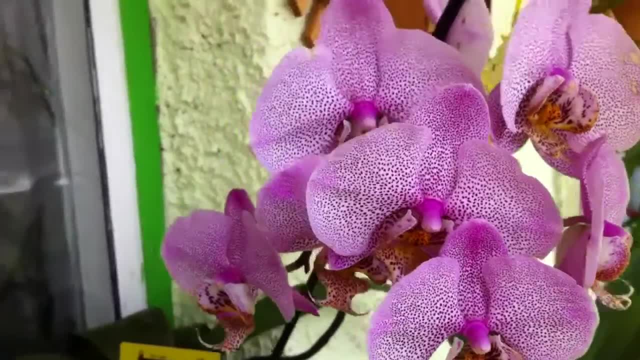 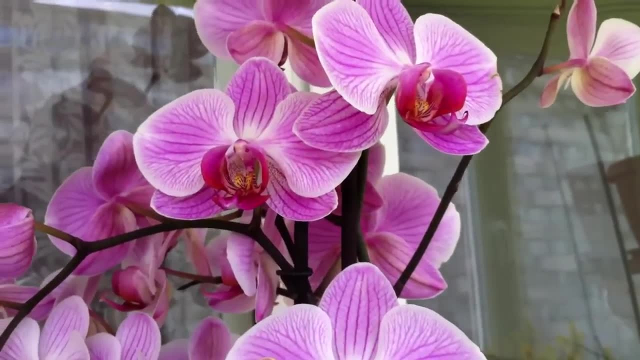 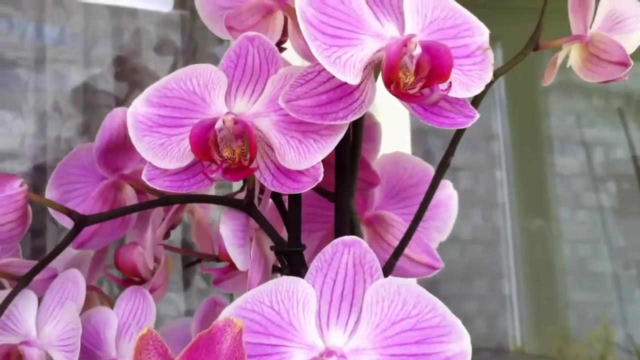 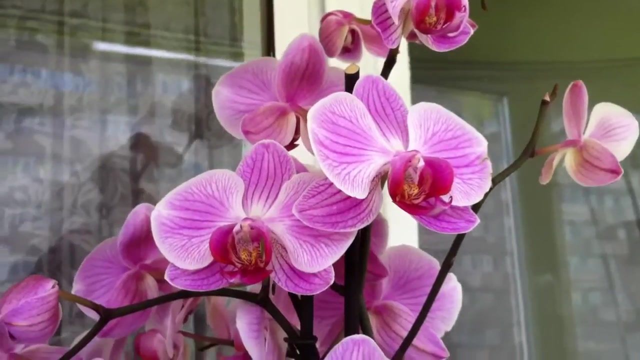 absolutely gorgeous. This one is actually a pretty common Phalaenopsis to find, and I saw it first in one of Suniti's videos. I think it's the same type. She had a beautiful, beautiful re-bloom out of her and actually she won a prize, So I'm hoping I can do the same with 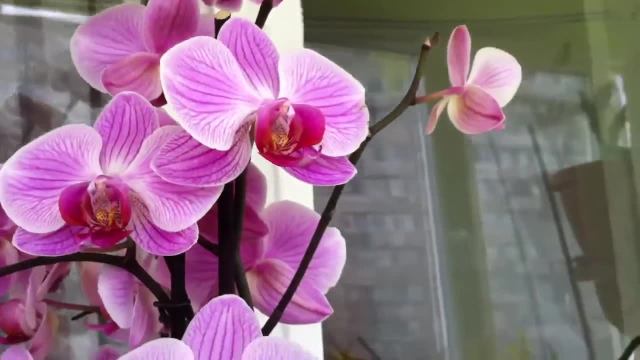 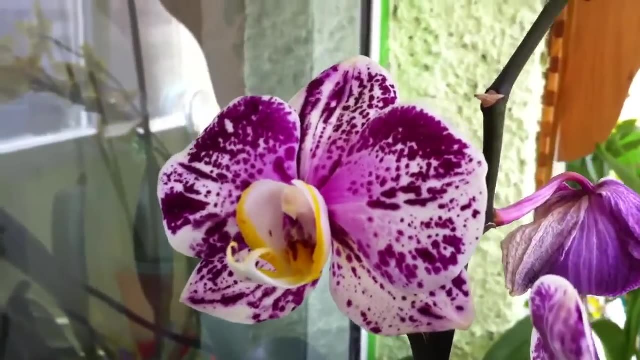 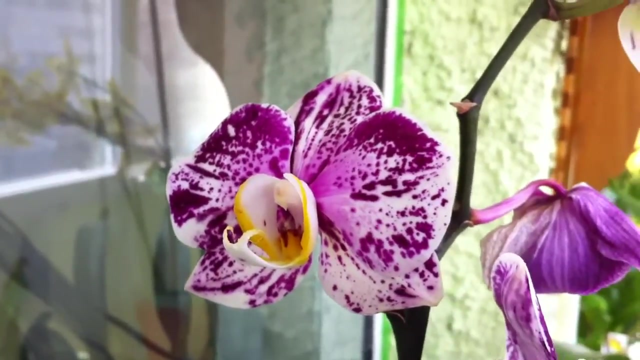 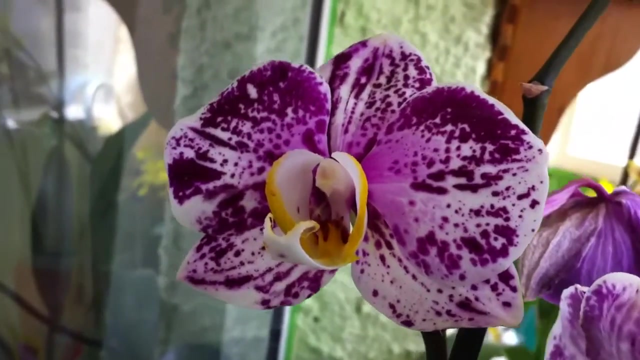 my orchid because I really like the color. This one is a more rare, let's say variety, because this is the only time I saw her in the store and I bought it instantly. She looks like a painting with smudged colors. I think she's lovely. 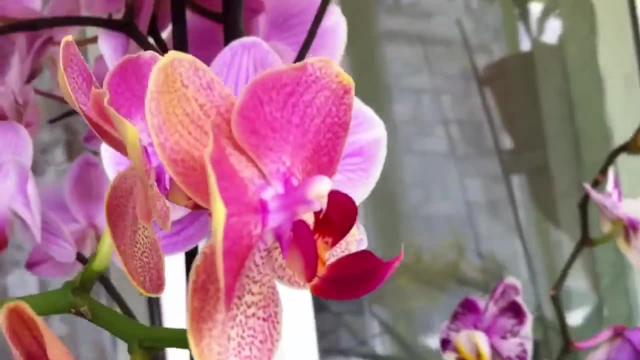 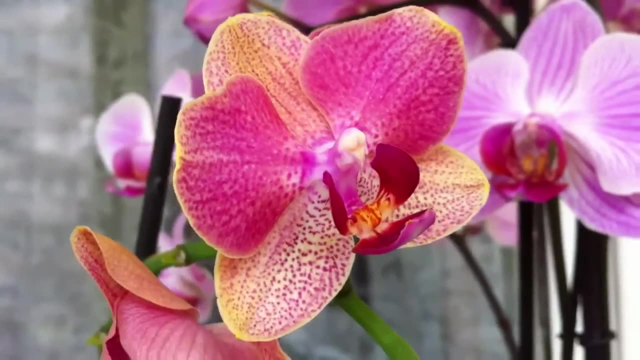 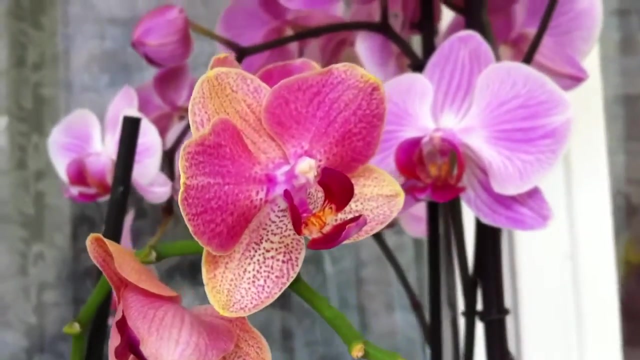 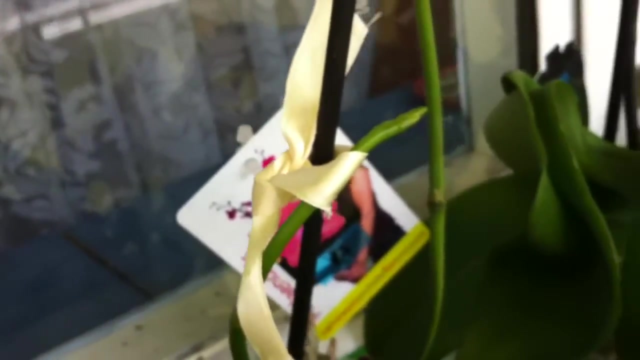 This one again. I don't know her name, but she has some yellow color along with dark red. Unfortunately she's dropping her flowers, but she has a secondary spike and a primary spike developing, So I'm happy I'm going to see the blooms again. 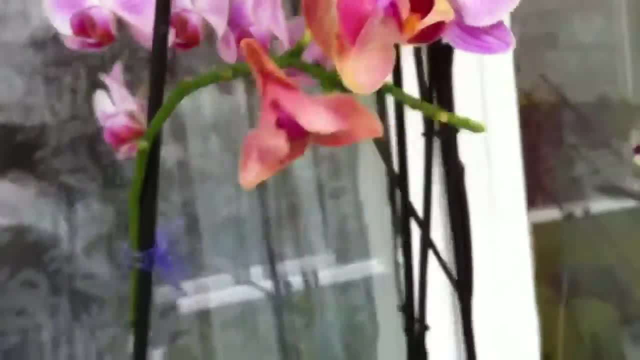 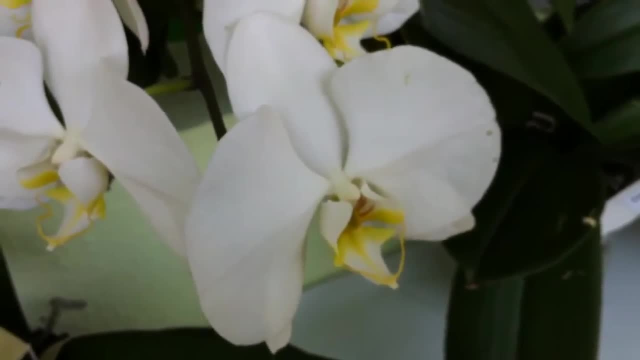 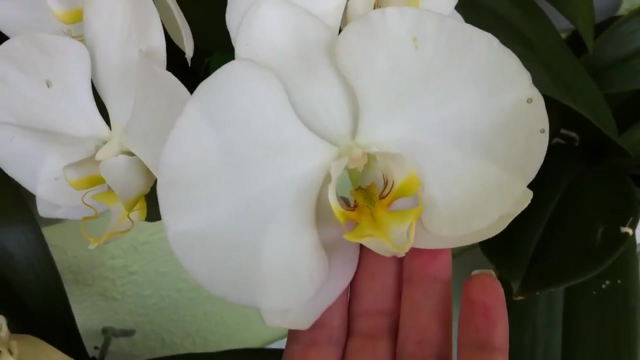 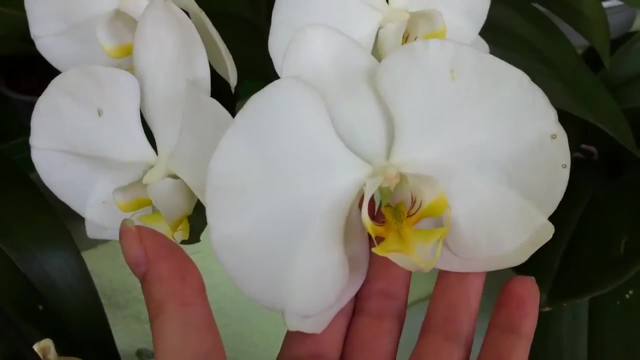 You know my beautiful white princess already. You can find this variety with a dark red lip. I don't know why I didn't buy that variety yet, but I will when I see it, because I absolutely adore the big flowers and I didn't see any other orchid. 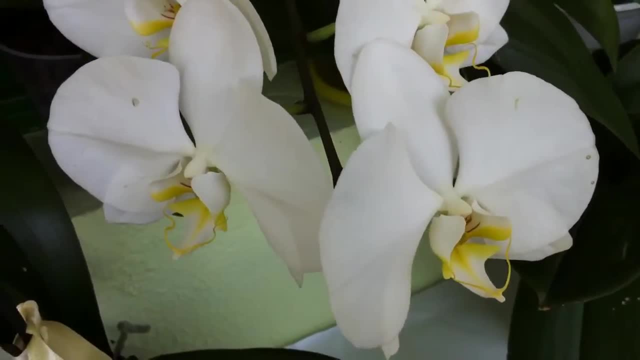 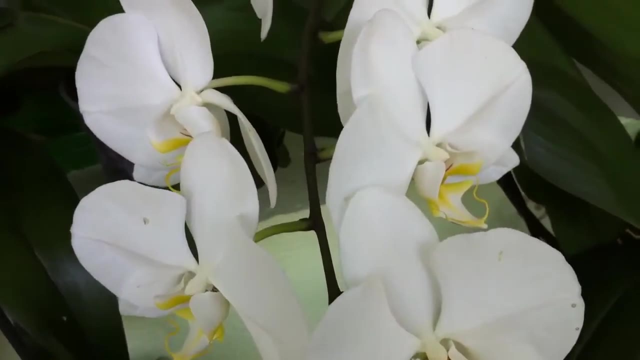 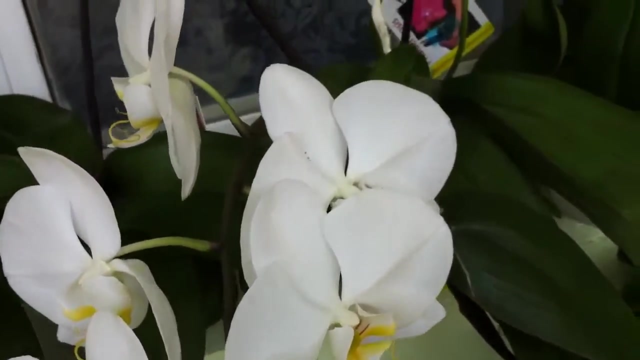 I'm really proud of the shingling I did on this one. It took me a while to understand that the spike heads towards the light and I should not move an orchid that is in spike. Don't move your orchids when the spike is developing and you can get this beautiful. 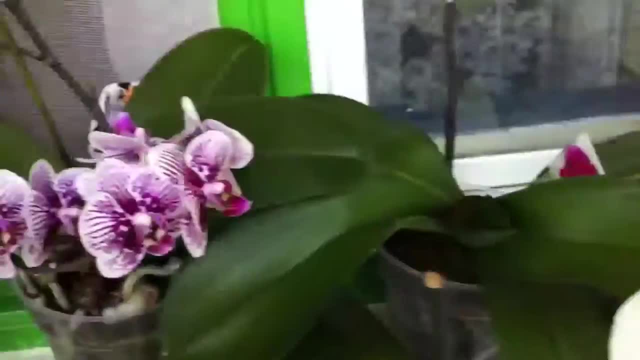 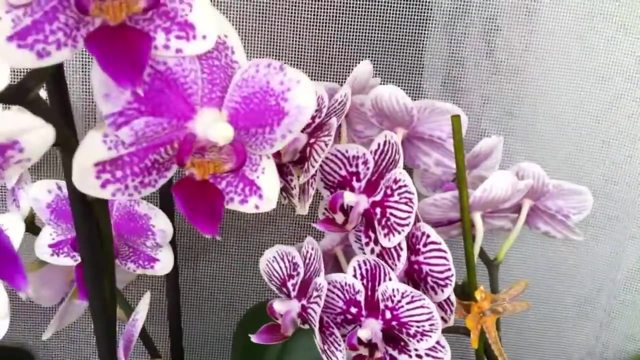 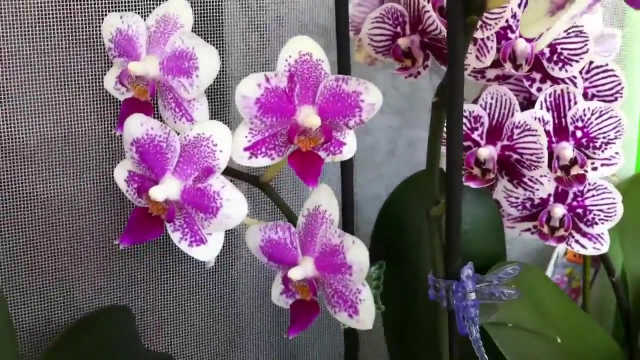 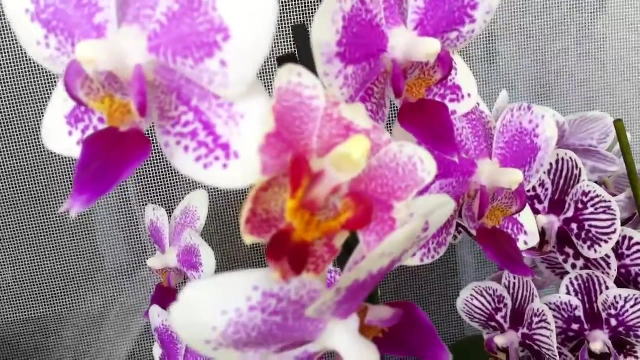 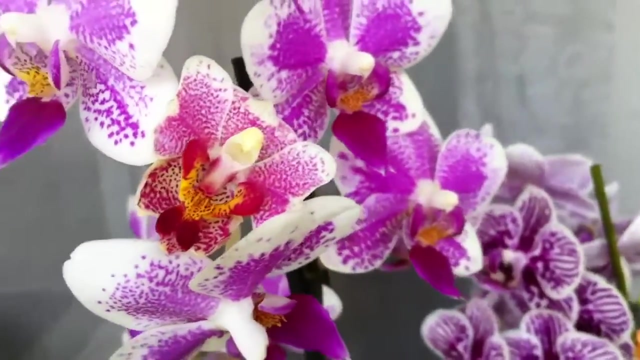 shingled appearance. You also know this one. She is actually called Little Zebra and I think it is very fitting for her. This one I didn't identify yet, but she is gorgeous And she just produced a deformed flower. It's nothing to worry about. Phalaenopsis sometimes do this. It doesn't mean anything. 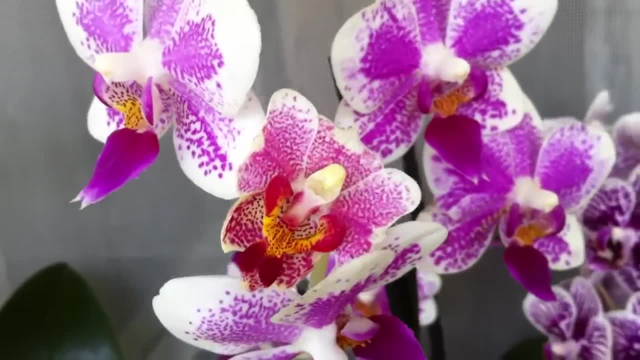 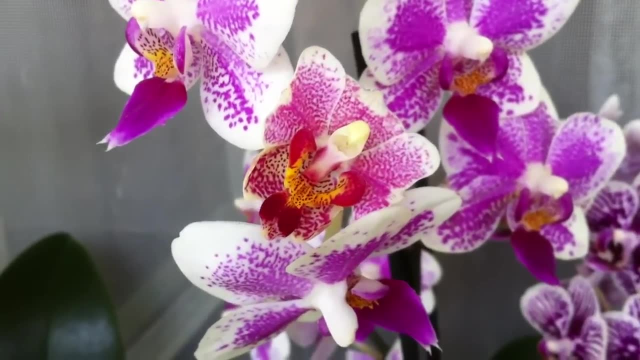 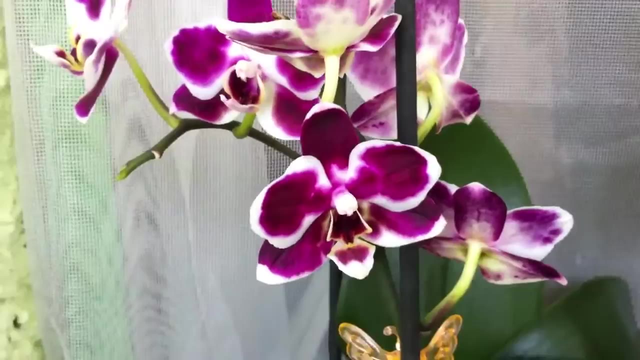 It just looks funny And excellent. Actually, I just noticed now it definitely looks like a butterfly. I guess that's why they call them the moth orchids. You might also know this one. Her name is Sogo Lovely, as far as I've been able to tell. 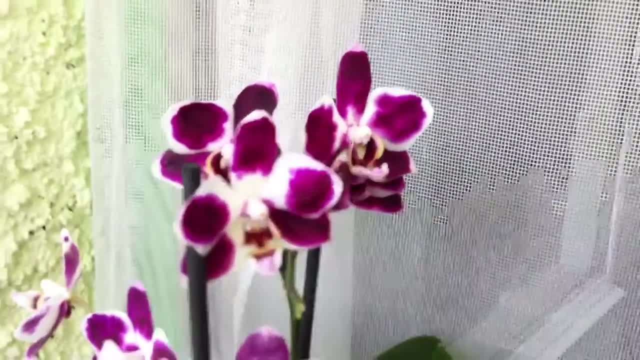 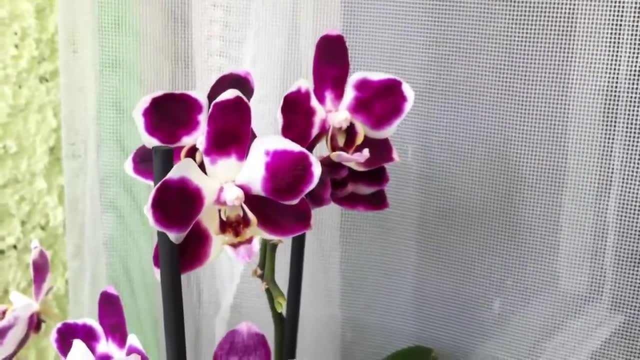 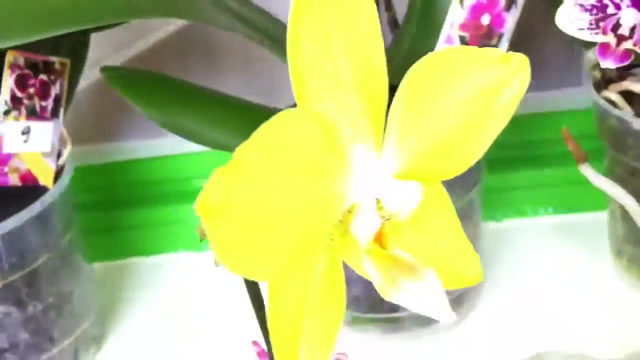 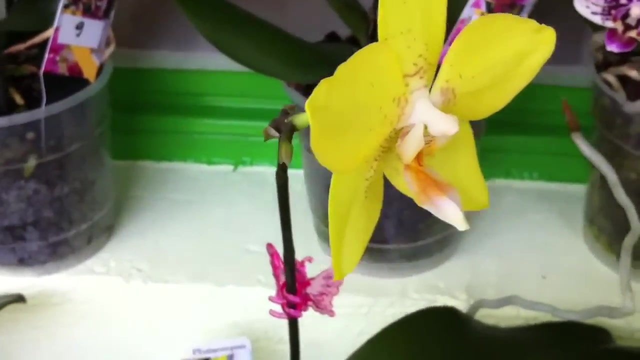 And what's nice about her is that on the same flower spike she has different colored flowers. This sometimes happens with Phalaenopsis, so it's great to have different flowers on the same flower spike. This yellow beauty, unfortunately, is left with one single flower. she used to have more. 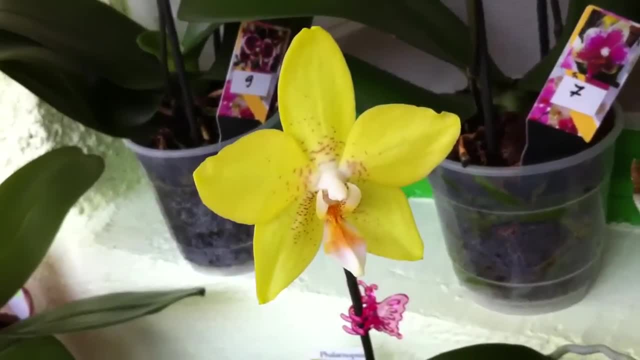 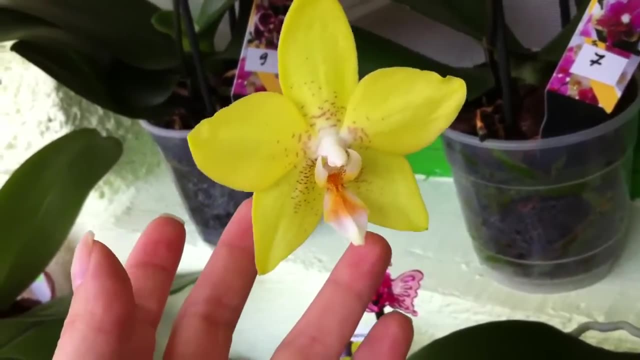 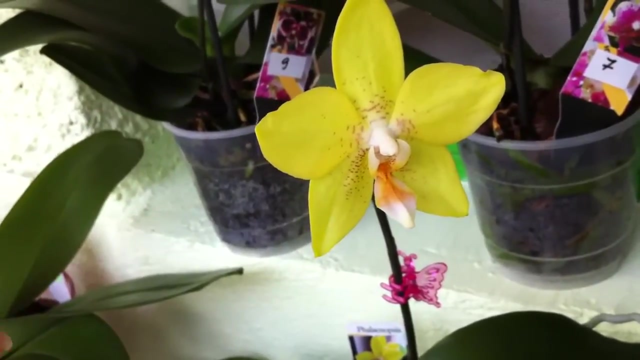 But she's beautiful. This is the first time she re-blooms for me. I have her since last year and I absolutely love the color and the orange light. I also like that. she has kind of pointy petals. they're now round. 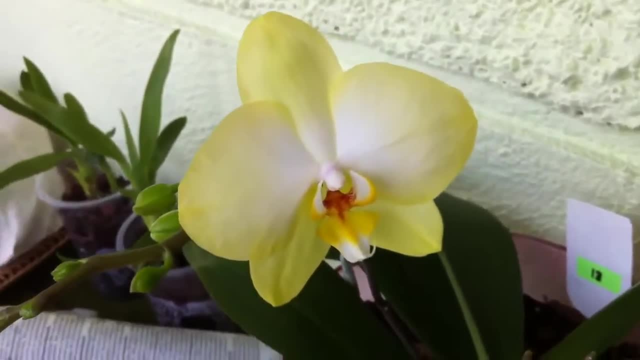 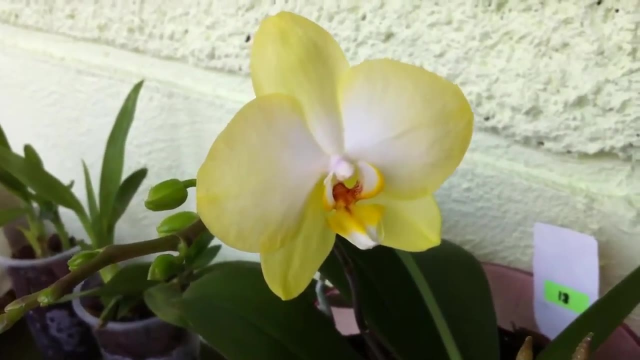 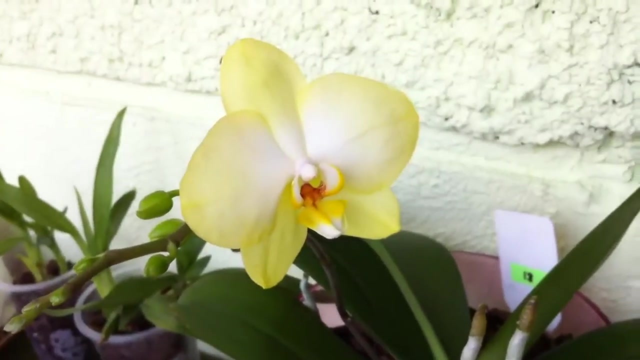 And the last Phalaenopsis that I have in bloom right now is this one, which is by far the most interesting orchid I have. It doesn't look interesting, but I'll tell you why I find it interesting. This is my oldest Phalaenopsis. 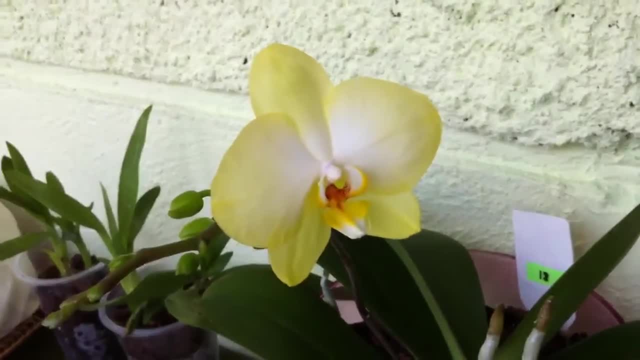 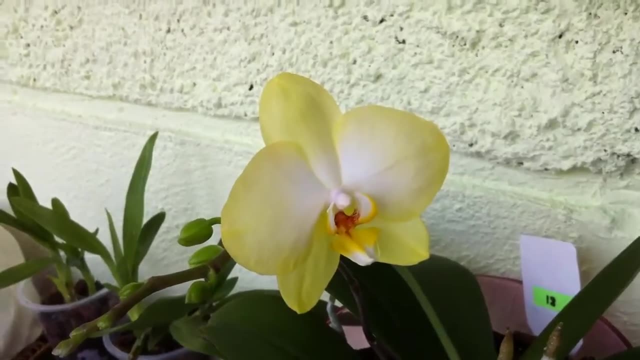 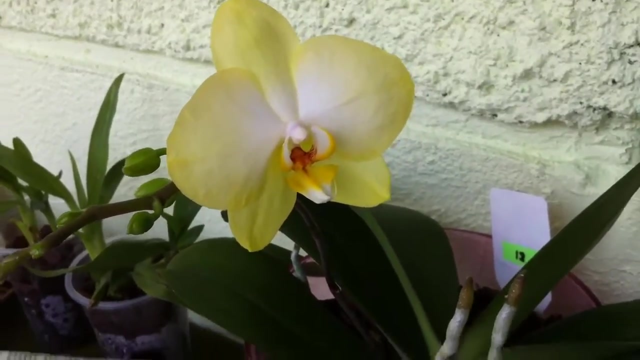 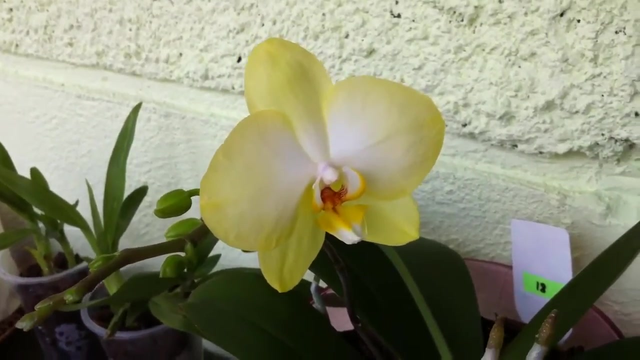 She has three years with me And I actually gave her to my mom And we both remember her as being completely white and now she's yellow. Now the reasonable explanation would be that we didn't remember correctly, But if not, it might mean that she has a yellow hybrid in her genes and she now decided to.